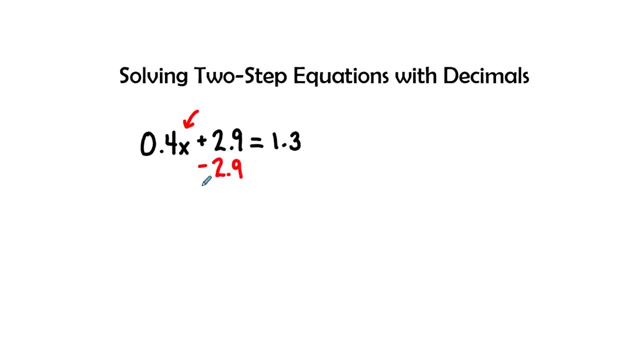 negative 2 and 9 tenths. Once I add a negative 2 and 9 tenths, this is going to equal 0. And I have to remind myself that what I do on one side of the equation is that I add a negative 2 and 9 tenths to the variable. So I'm going to 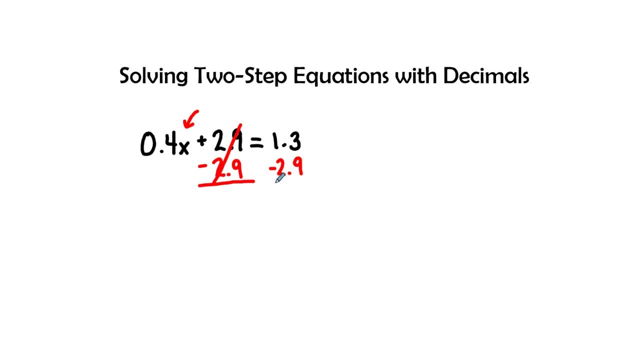 have to do on the other side of the equal sign. And there we go. When I go ahead and bring down, let's go change to black. I have 0 and 4 tenths x, keeping my equal signs in line with each other. Now I have a negative 2 and 9 tenths plus 1. 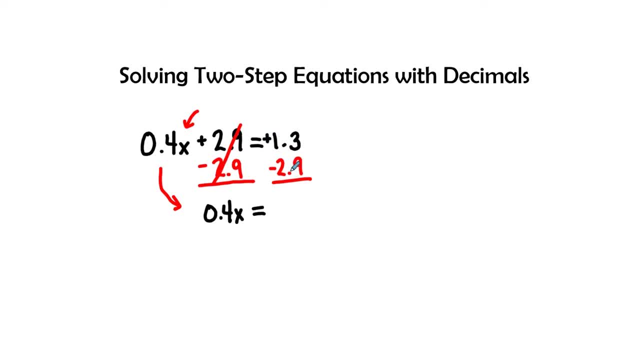 and 3 tenths, because this is a positive right here It gives me a negative 1 and 6 tenths. I could do some calculations off to the side. I can use a calculator. That is okay. Now for our next step. I see the x still has 4 tenths attached to it And we 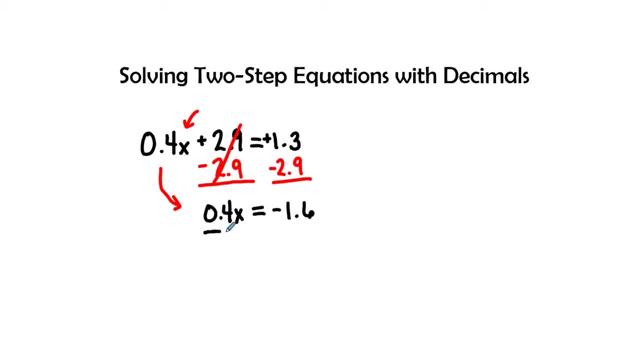 said earlier that it was multiplication, And to find the inverse, I am going to go ahead and divide by 4 tenths on both sides. Now, 4 tenths divided by 4 tenths is 1.. And so I have 1 x equals. 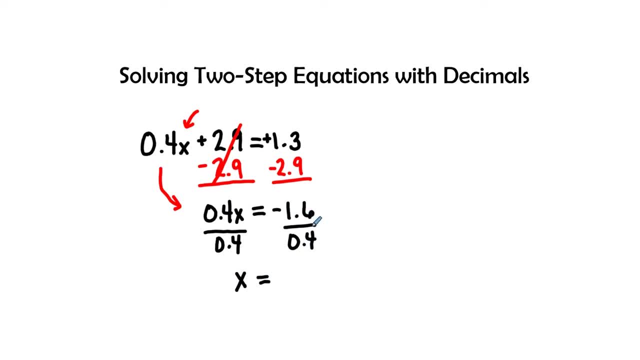 and then a negative 1 and 6 tenths divided by 4 tenths. I'm going to say how many 4 tenths, because the opposite of division is multiplication. So I could go backwards and I can say I have 4 tenths, Another 4 tenths is 8 tenths. If I add another 4 tenths is: 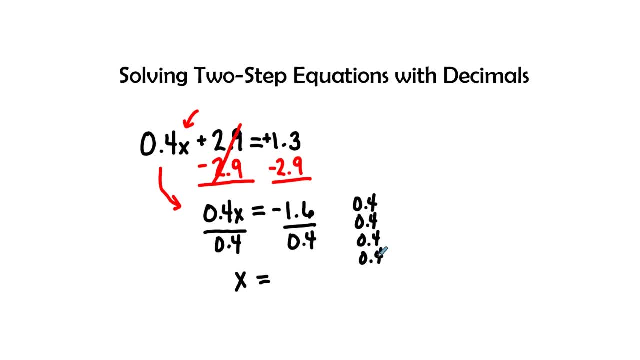 1 and 2 tenths And this is 1 and 6 tenths. So it's 1, 2, 3, 4.. So there are in 4 tenths. there are 4, 4 tenths and 1 and 1 tenth, 1 and 6 tenths. 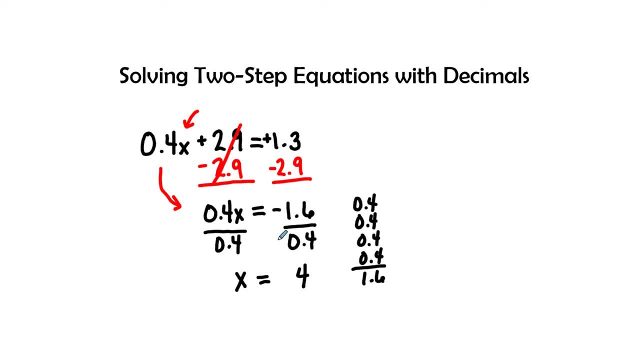 Excuse me, So I have a negative and this is a positive. So a negative and a positive is a negative. Let's go back and check our work, just to double make sure, double check and make sure that we got the correct answer. So I'm going to write this problem again: 0 and 4, 0.4 x, or.